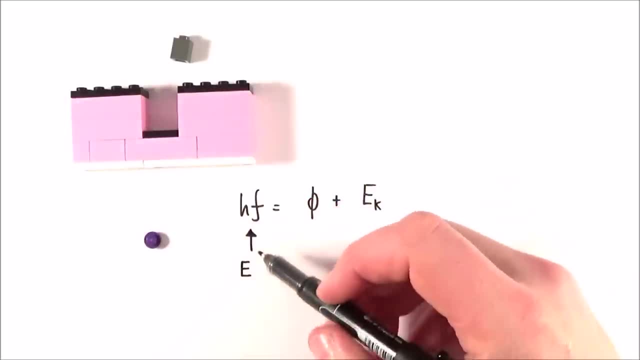 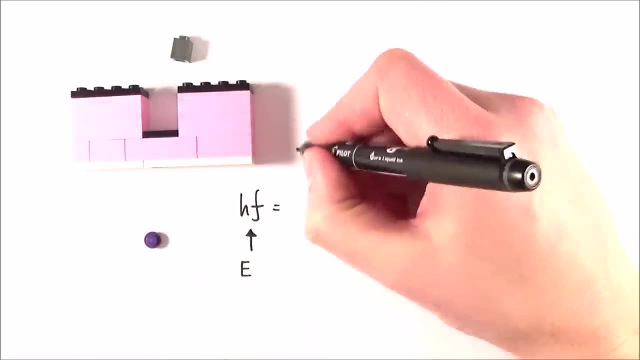 of the equation hf. this comes from the fact that we can look at the energy of the photon and relate that to the frequency of the associated wavelength. We then have this bit here which is what we call the work function, And this work function is effectively a measure of 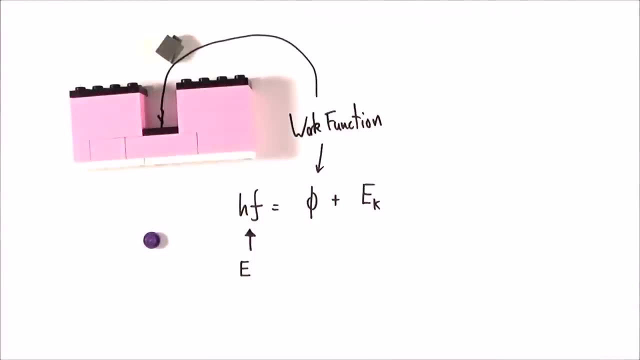 the size of that hole that the electrons are actually coming out of. And then, finally, this is the maximum kinetic energy that the things could have, So ek being the kinetic energy which obviously we know is equal to a half mv squared, And you can often find 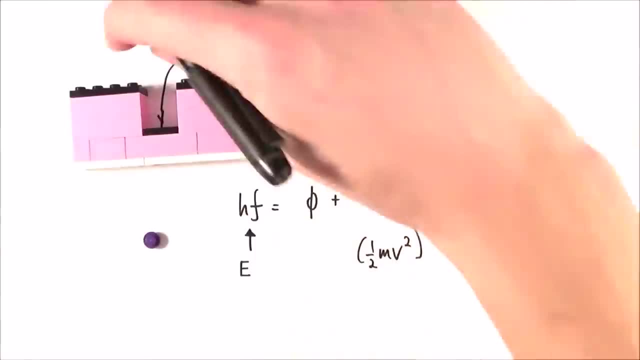 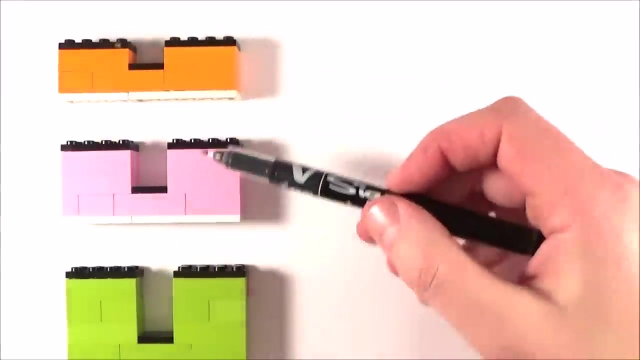 the mass of the electron in your data book. So this is how much energy the electron goes flying off with after it's been liberated from that atom. And this equation here is known as Einstein's equation. What we find is that different materials have a different size energy gap And from the equation we just had, where hf is equal, 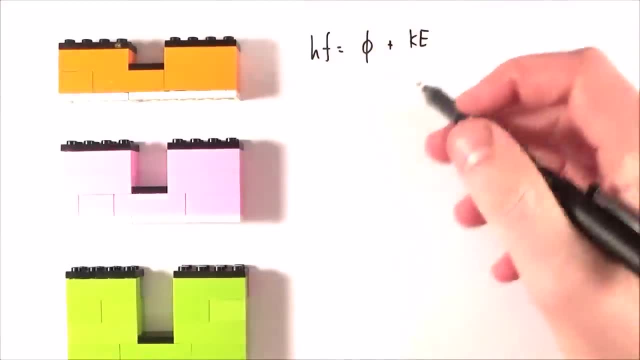 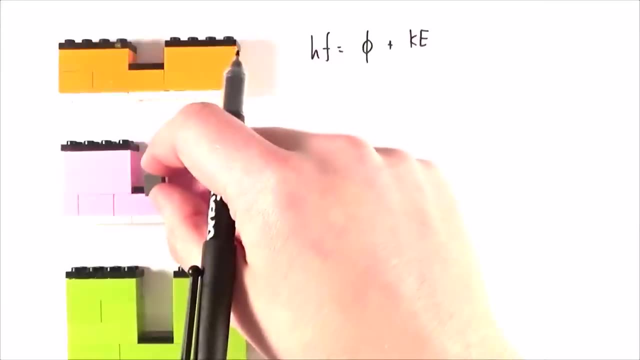 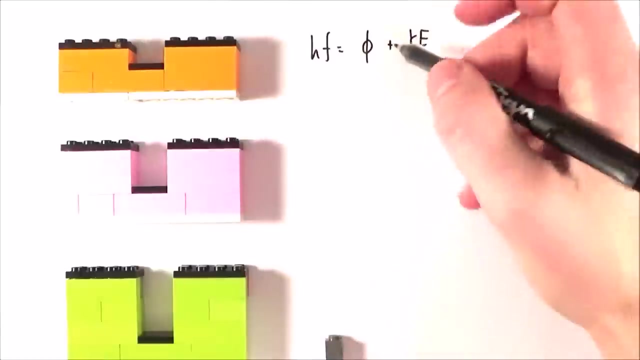 to the work function plus the kinetic energy, either ek or ke, of those particles. we can look at maybe, a scenario where we just about get the electron out of that energy well onto, effectively, the very edge of that material, And what we can then say is that the kinetic 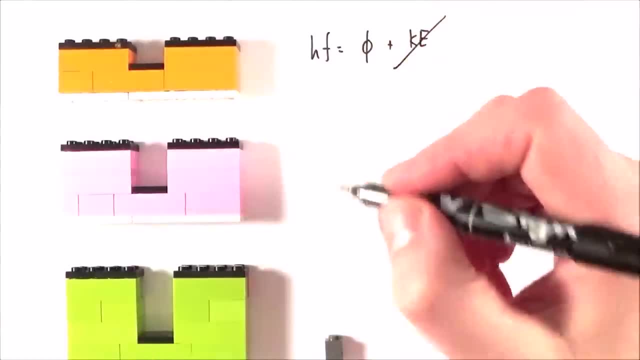 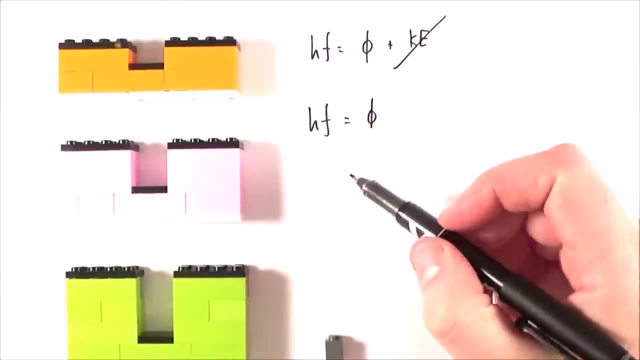 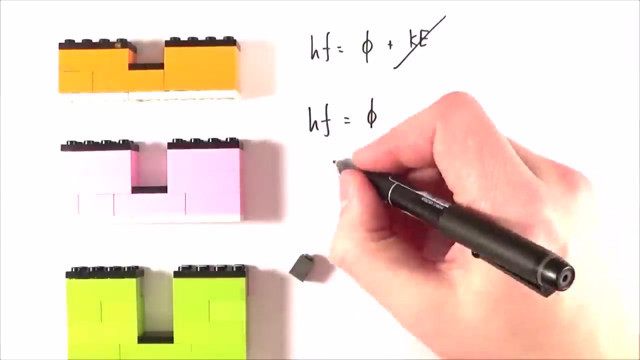 energy is going to be zero, And what we can look at then is something called the threshold frequency. So we can say that hf is equal to the work function, And, provided we're looking at the minimum frequency of the instant radiation, or the minimum energy of that photon, we can 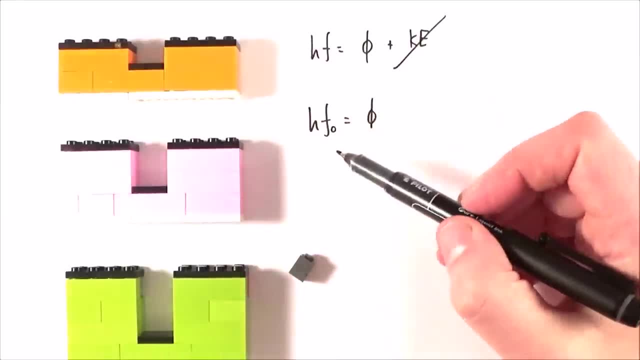 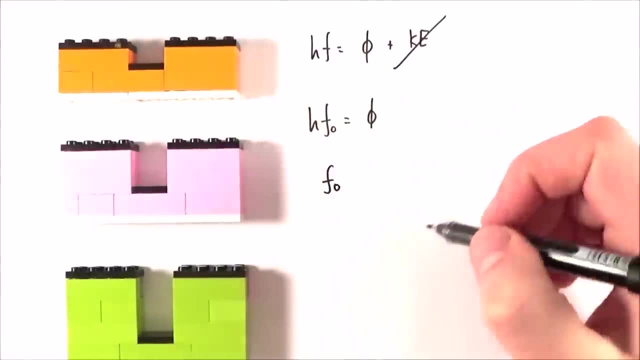 then call this f0 or f0. And that stands for the threshold frequency. So this threshold frequency, the minimum frequency at which we start to liberate the electrons, is going to be equal to the work function of that material divided by Planck's constant. And 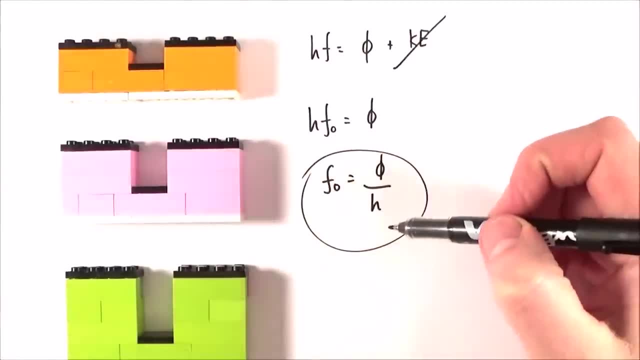 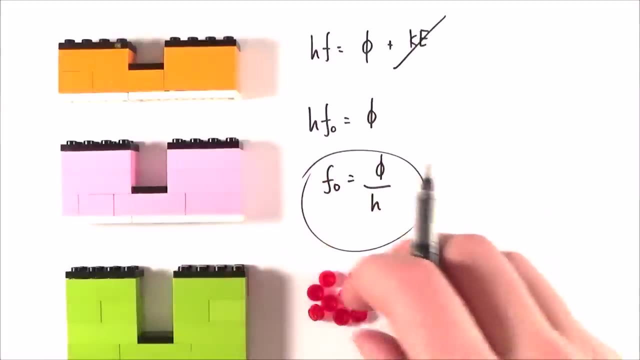 this thing. here is the real crux of why the photoelectric effect is important and has something to do with quantum physics, Because it doesn't matter how many red photons you have landing on that or instant on that piece of metal If all of these are below the threshold.